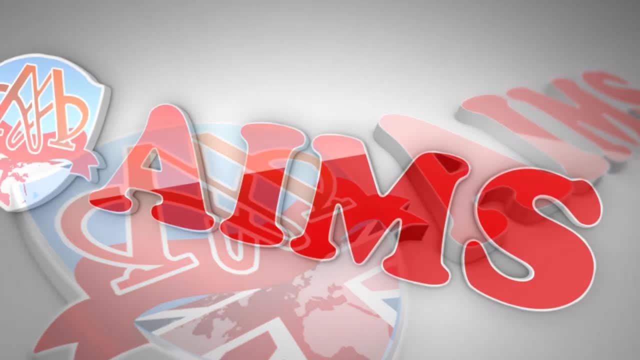 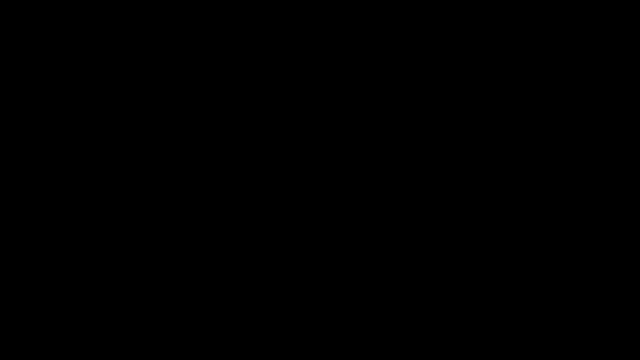 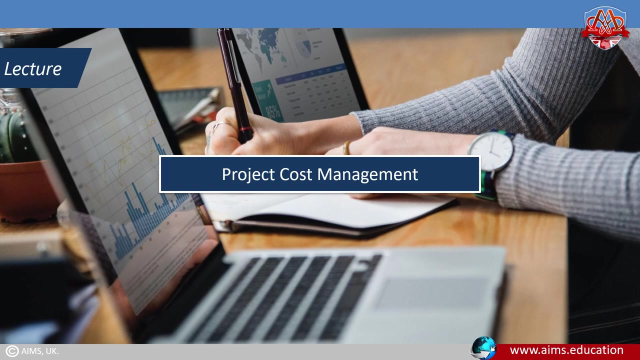 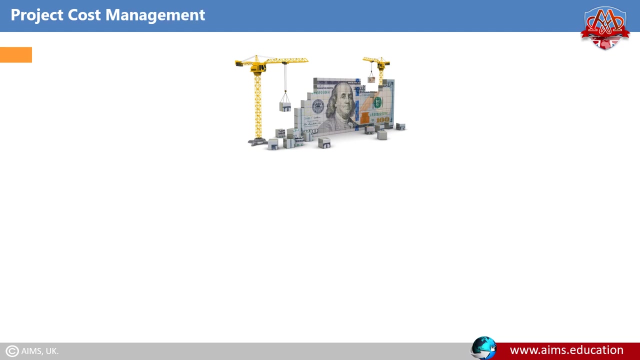 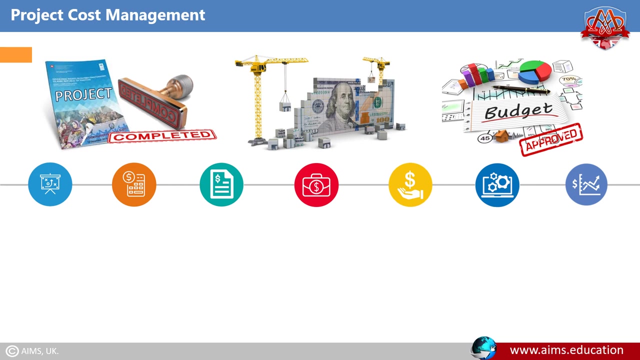 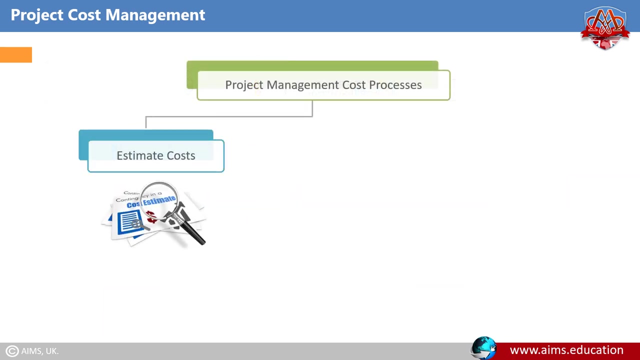 Project Cost Management. Project cost management includes the processes involved in planning, estimating, budgeting, financing, funding, managing and controlling costs so that the project can be completed within the approved budget. The below figure gives an overview of project cost management processes. Estimate costs is the process of developing an approximation of the monetary resources. 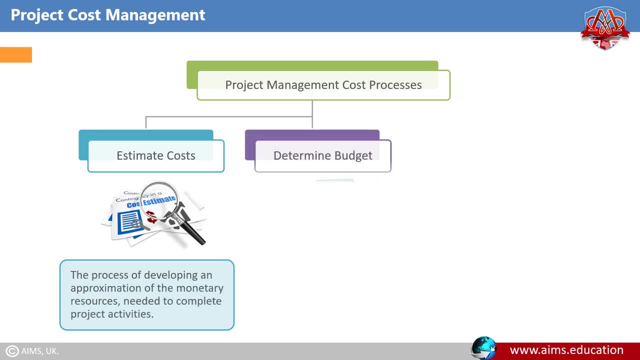 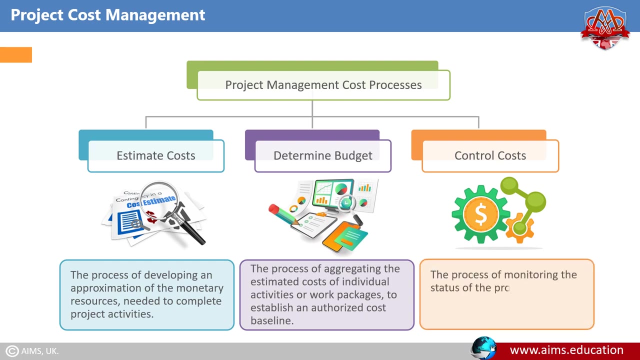 needed to complete project activities. Determine budget is the process of aggregating the estimated costs of individual activities or work packages to establish an authorized cost baseline. Control costs is the process of monitoring the status of the project to update the project costs and managing changes to the cost baseline. 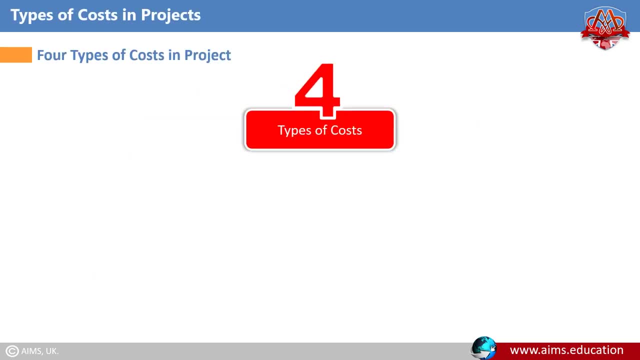 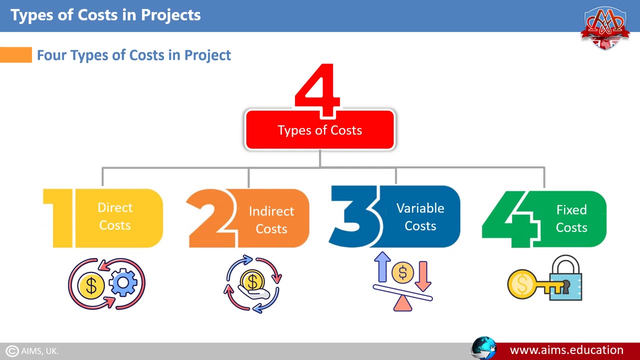 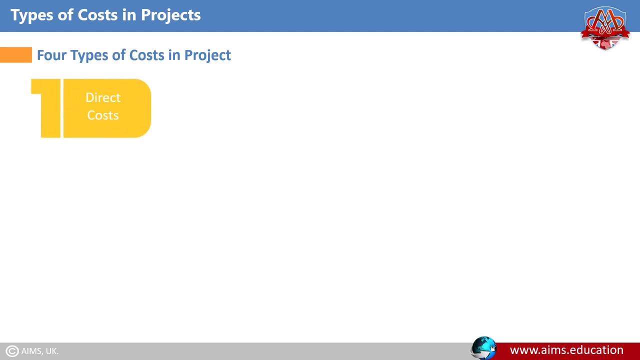 Types of Costs in Projects. There are four types of costs in projects – direct costs, indirect costs, variable costs and fixed costs. Direct Costs: Direct costs are the expenses that are billed directly to the project. They can be traced back to a product and can be measured, and. 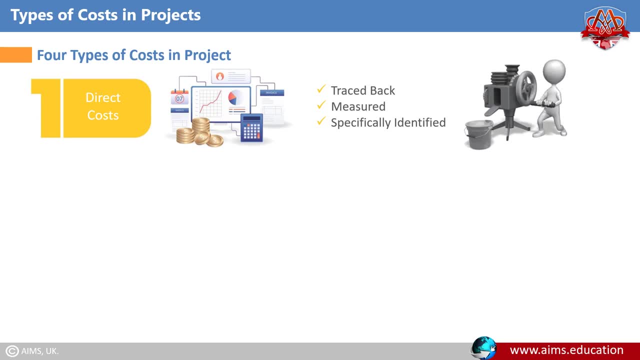 they are specifically identified by their objectives. Examples of direct costs are direct materials, direct labor, use of equipment, use of facilities, number of employees and consumption of services- Indirect Costs. Indirect costs are not directly identifiable, They are not directly related to the project product and they belong to the core supporting. 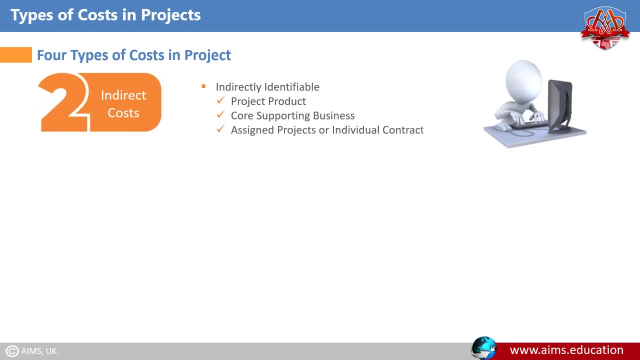 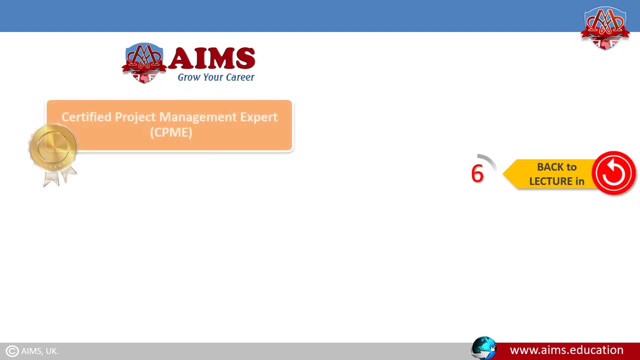 business, but cannot be directly assigned to projects or individual contracts. Examples of indirect costs are fringe benefits, indirect manufacturing expenses, general indirect expenses and general and administrative expenses. าμς is a globally recognized and an accredited Institution. We offer certifications, diploma, MBA and Shipbuilding program and program management. 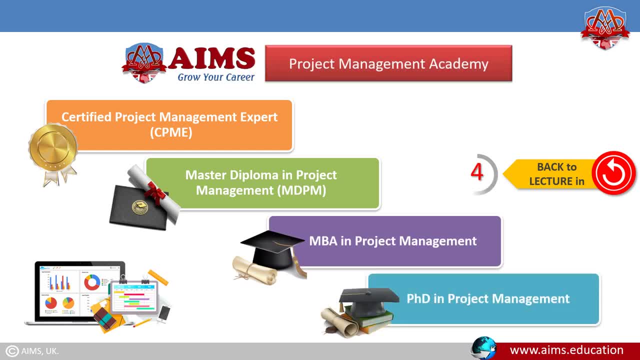 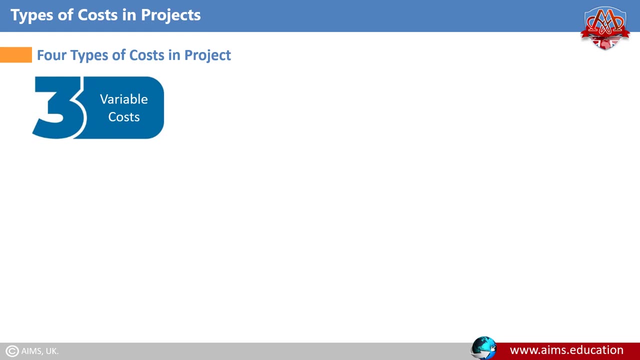 through an online and self-paced learning system. Variably Costs: Variable costs vary as changes in the production are implemented. In other words, they are reduced in scheduleえて. products are implemented to, dlatego they are in order. Bella Pinterest open the events to create times themselves. variation costs are said to be variable as changes are implemented from time to time. in other words, There are many other variations: evaluation to and fromirrels, whilst 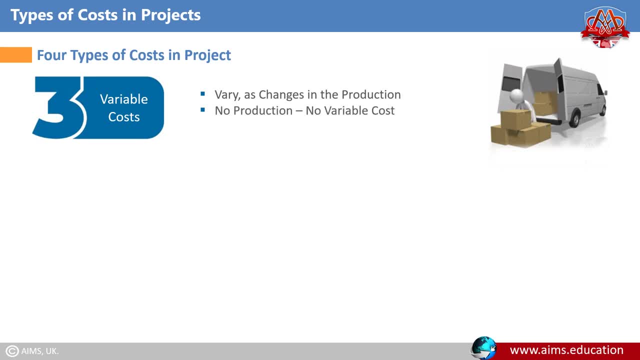 is no variable cost when there is no production. Examples of variable cost are running expenses of equipment and materials, performance bonuses, freight and sales commissions, Fixed costs. Fixed costs remain constant and they are independent of the amount of work performed. In other words, fixed costs remain the same even when the production line is null. 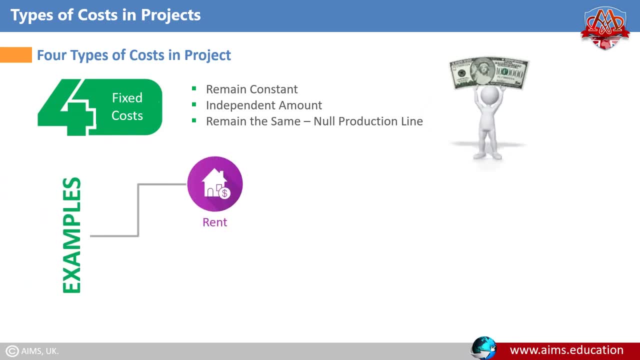 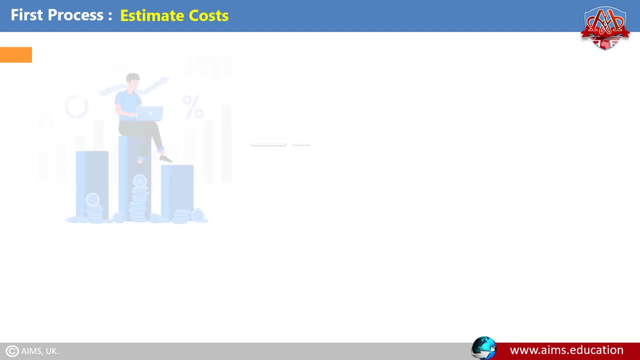 Examples of fixed costs are rent, depreciation, administrative team salaries and general expenses. Understanding the first process, Estimate costs, It is the process of developing an approximation estimate and it is used to calculate the cost of resources, materials and human, which are: 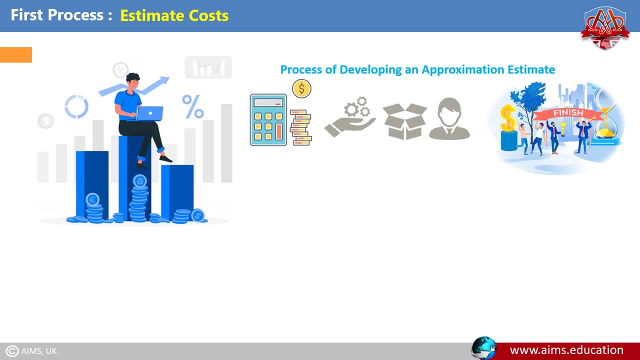 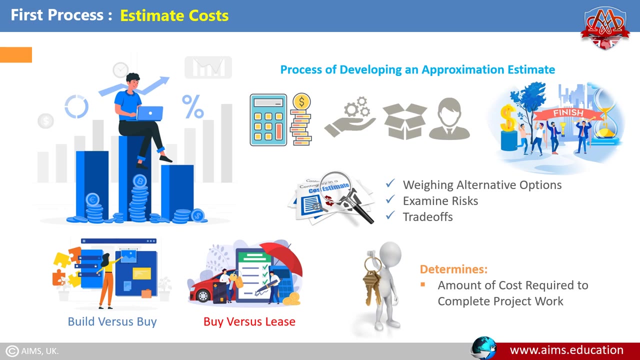 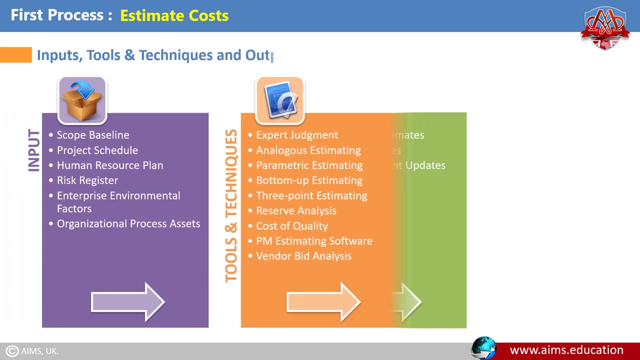 necessary to complete the project activities. Estimate costs also include the cost of weighing alternative options and examining risks and trade-offs, For example, build versus buy or buy versus lease. Key benefit: It determines the amount of cost required to complete project work. The inputs, tools and techniques and outputs of the cost estimate process. 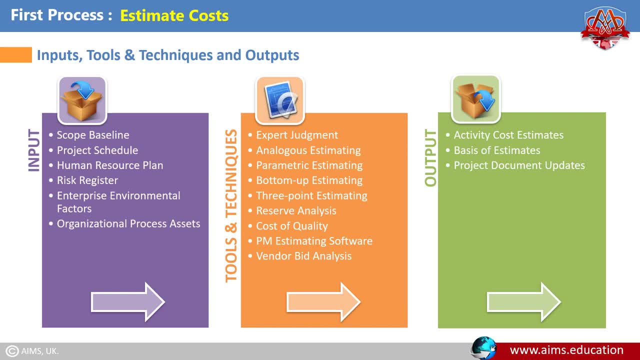 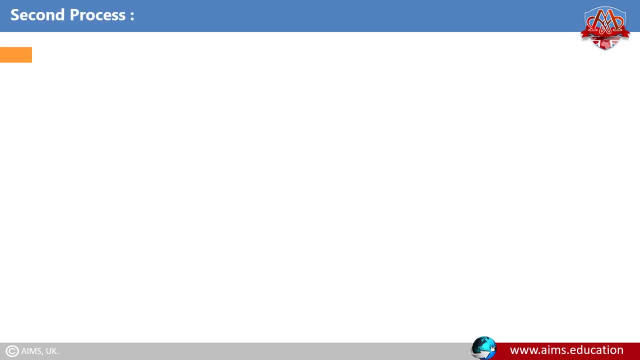 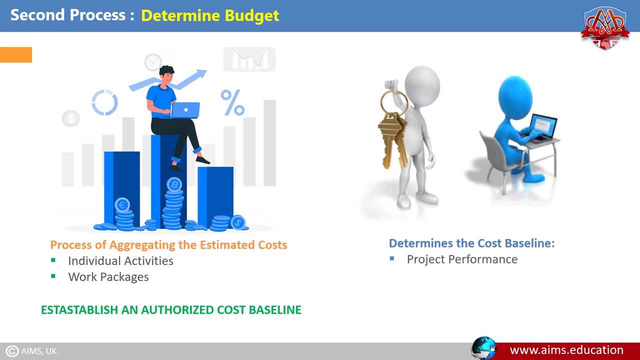 are depicted in the following figure. Understanding the second process- Determine budget- It is the process of aggregating the estimated costs of individual activities or work packages to establish an authorized cost baseline. Key benefit of this process is that it determines the cost baseline against which project performance can be monitored and controlled. 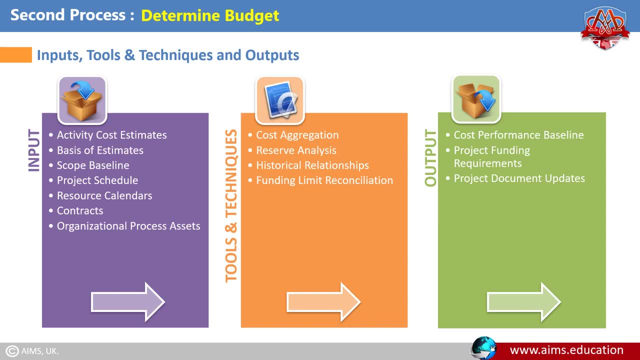 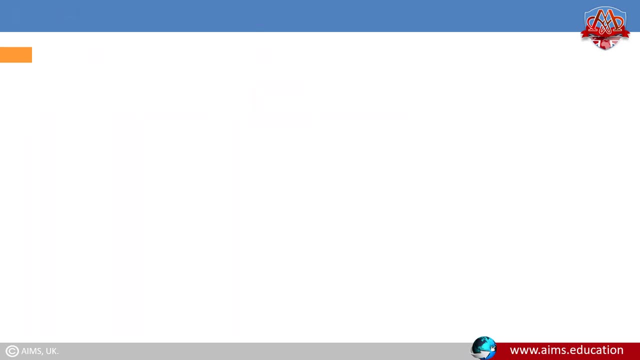 The inputs, tools and techniques and outputs of the determined budget process are depicted in the following figure: Shit Translation. Now let us understand control costs. These processes monitor the status of a project in order to update the project costs. It allows project managers to manage the changes in the cost baseline, if present. 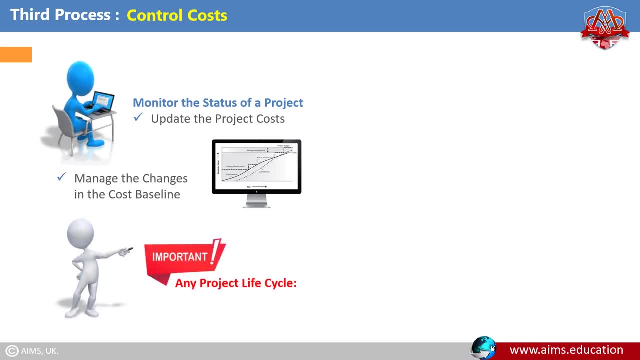 It is important to note that in any project life cycle there will be changes in the cost Key Benefit. It provides the means to recognize variance from the plan, particularly on cost, so that they can take the appropriate corrective action to reduce the risk. 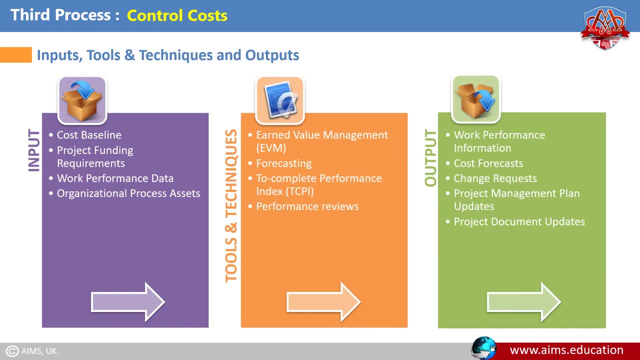 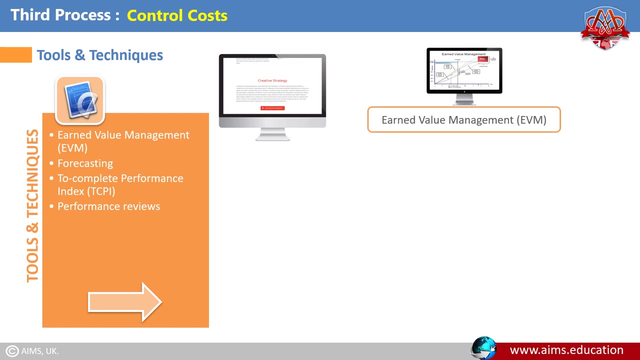 The inputs, tools and techniques and outputs of the control costs process are depicted in the following figure. Tools and techniques for control costs. Tools and techniques for control costs are earned value management or EVM, forecasting to complete performance index or TCPI and performance reviews. 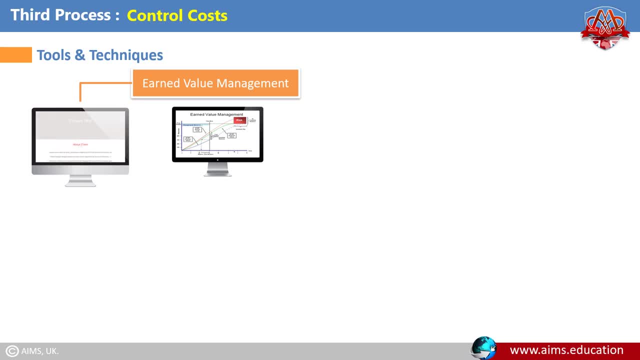 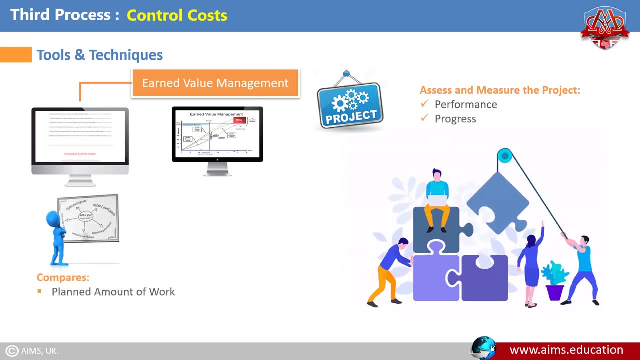 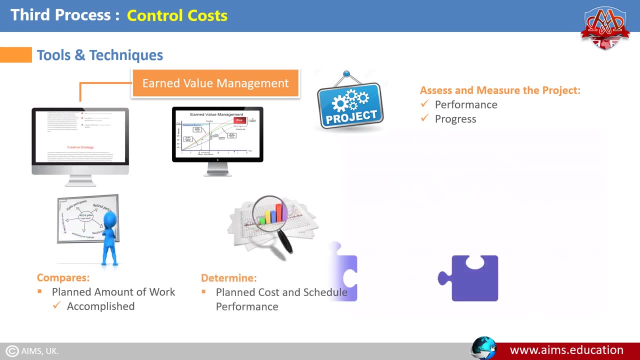 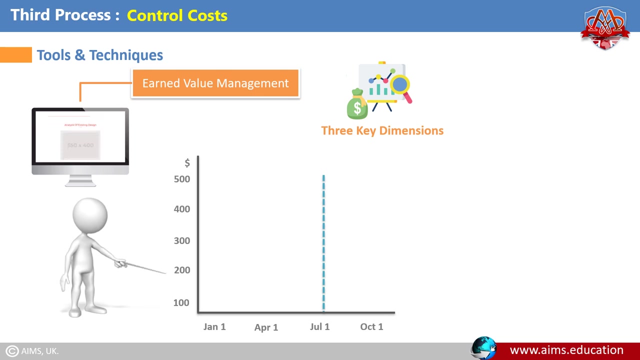 Earned value management. This technique helps the project management team to assess and measure the project performance and progress. It compares the amount of work that was planned with what was actually accomplished to determine if cost and schedule performance is as planned. Earned value management develops and monitors three key dimensions for each work package. 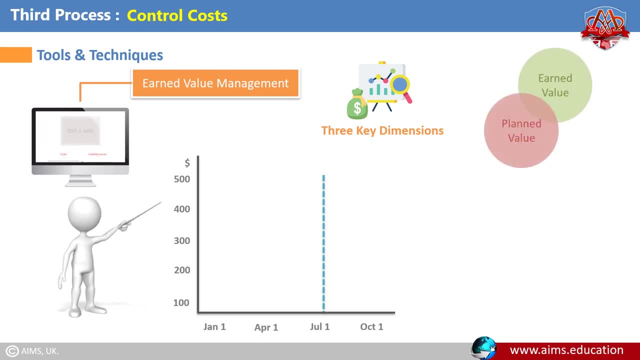 and control account Earned value, planned value and actual cost. Planned value represents the estimate value of the work planned to be done. Earned value represents the estimated value of the work actually accomplished and the planned cost to complete the work that has been done. 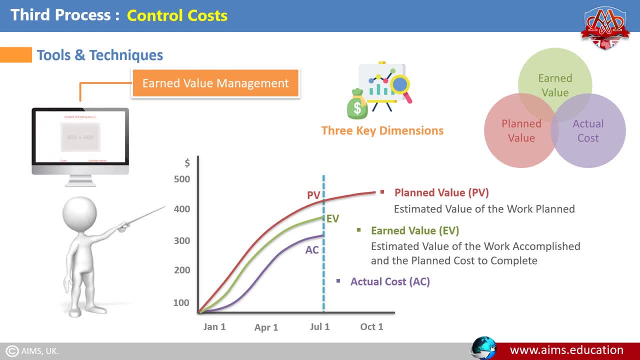 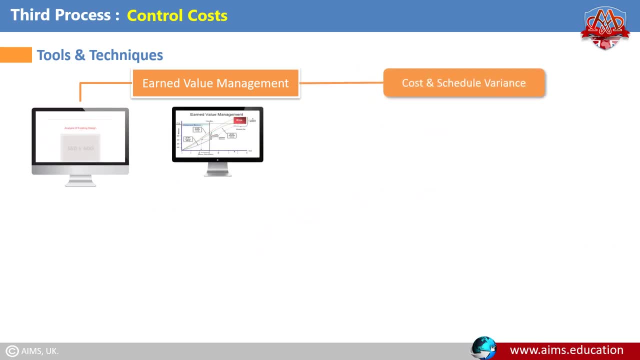 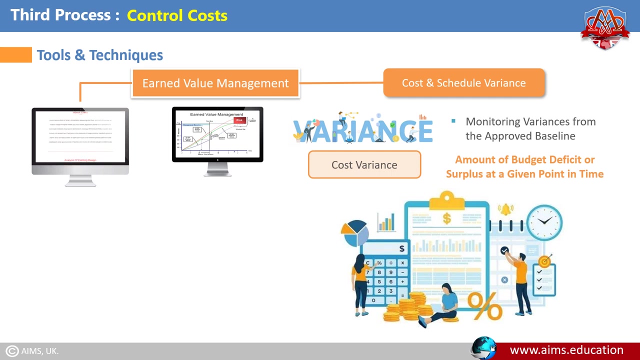 And actual cost or total cost is the cost incurred for the accomplishments of the work. Cost variance and schedule variance: Variances from the approved baseline are also monitored through cost and schedule variances. Cost variance: It is the amount of budget deficit or surplus at a given point in time and it is expressed 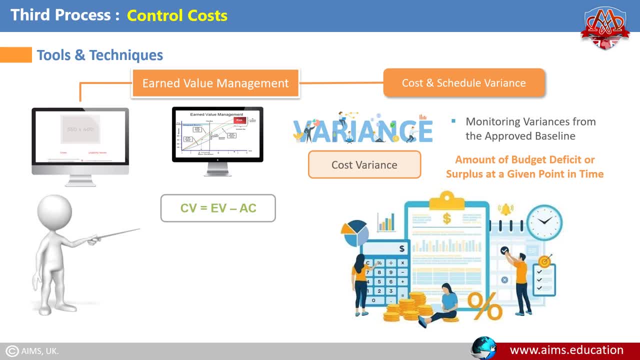 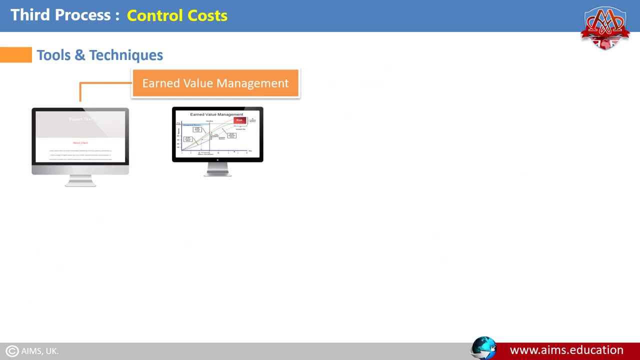 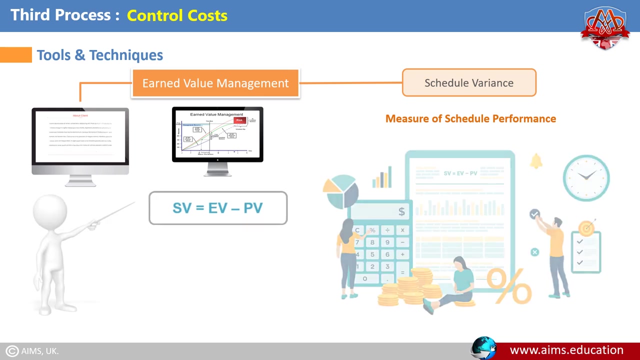 as the difference between earned value and actual cost. If the cost is higher than the budgeted amount, the resulting number is negative, and if the cost is lower than the budgeted amount, The resulting number is positive. Schedule variance: It is a measure of schedule performance and it's expressed as the difference between the 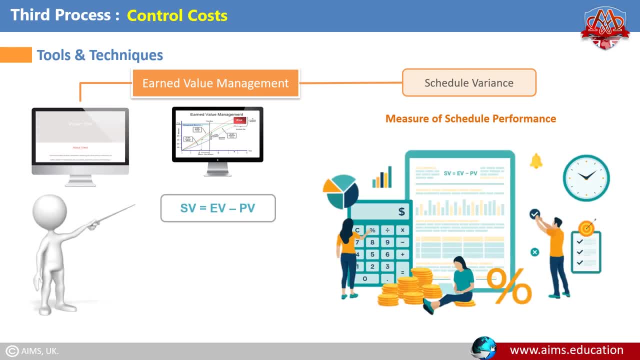 earned value and the planned value At the given point in time. if the project is ahead of the planned delivery date, the resulting amount is a positive number, And if the project is behind the planned delivery date, the resulting amount is a negative number. 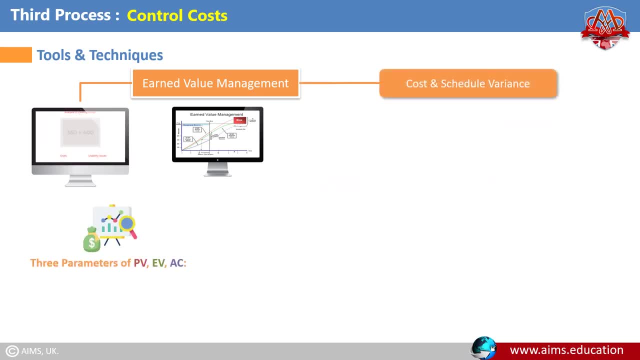 The three parameters of planned value, earned value and actual cost can be monitored and reported on both period-by-period basis, which is typically weekly or monthly, and on a cumulative basis. In the below figure, S-curves are used to display earned value data for a project that is performing. 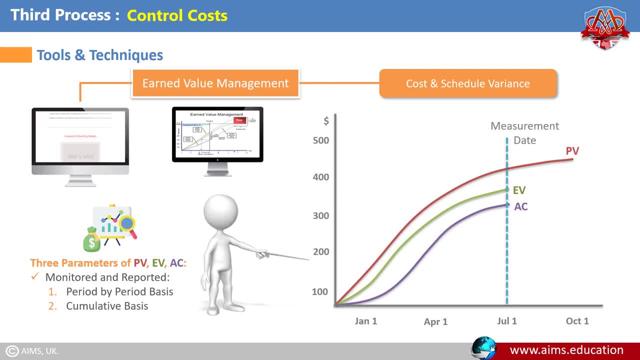 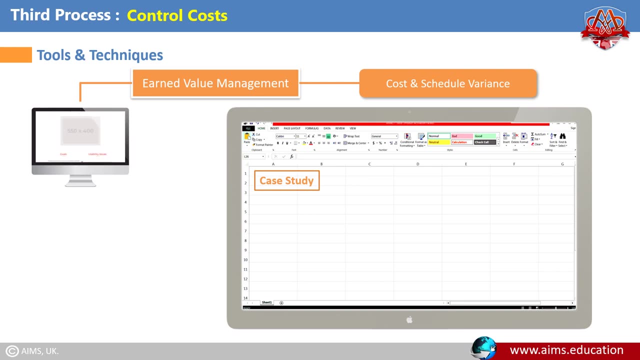 over budget and behind the schedule, and it also shows cost variance and schedule variance at any given point in time. Case study: Finding cost and schedule variance. Let us consider an example to find the cost variance and schedule variance of a given project. Suppose that for a project, the planned value is $400,, the earned value is $375, and the 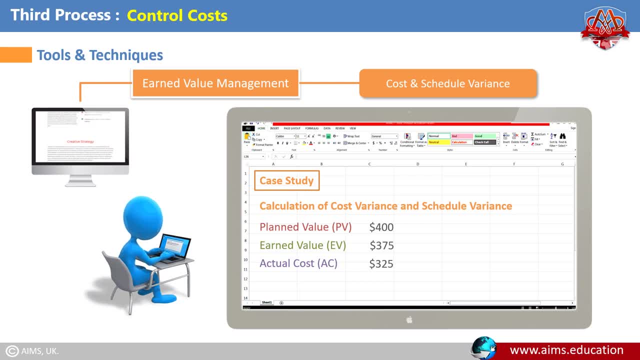 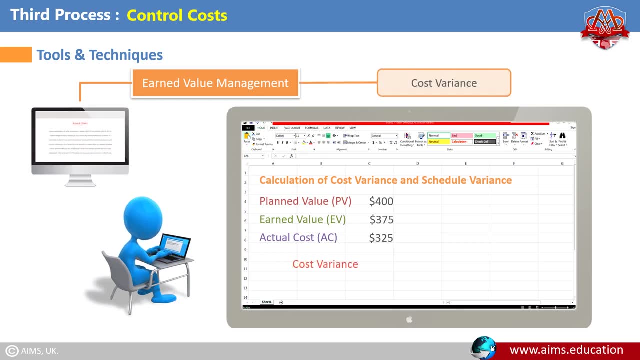 actual cost is $325.. Finding the cost variance. Using the formula of cost variance, we may calculate that the cost variance is $50.. Since the value of cost variance is positive, it means that we are spending less than the planned amount. Finding the schedule variance. 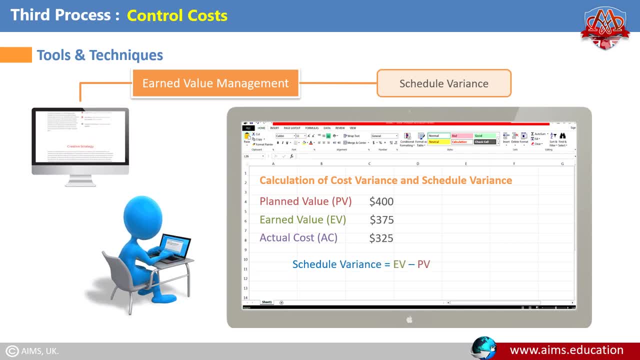 After using the formula of schedule variance, we may calculate that schedule variance is minus 25.. Since the value of schedule variance is negative, it means that our project is behind, And so the total cost is $35,000, which is an additional $50 for the completed project. 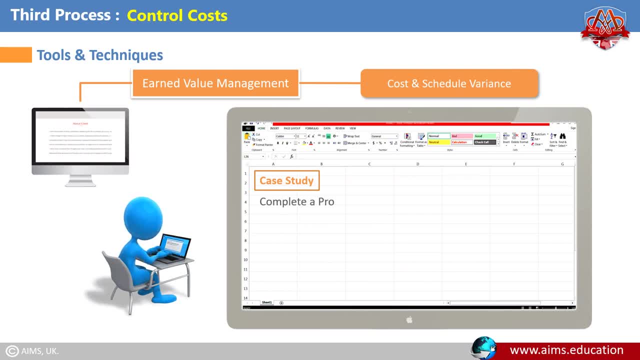 Case study. Suppose that you are required to complete a project in 12 months and the total cost of the project is $100,000. Finding the planned value, In our case, 50% of the work should be completed on completion of 6 months. 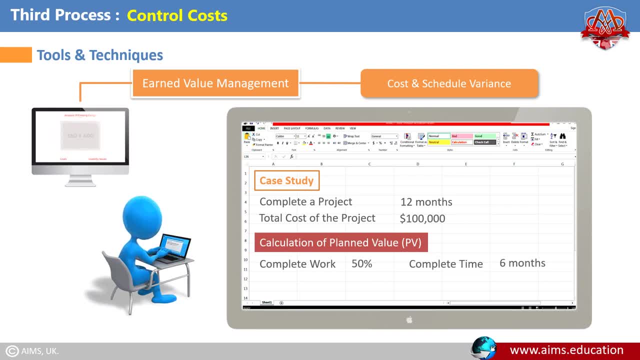 So the planned value of the project will be calculated as: planned value equals 50 % multiplied by $100,000. Or the current value of the project will be calculated as X, Or the planned value equals $50,000.. Finding the Earned Value: On completion of six months you find out. 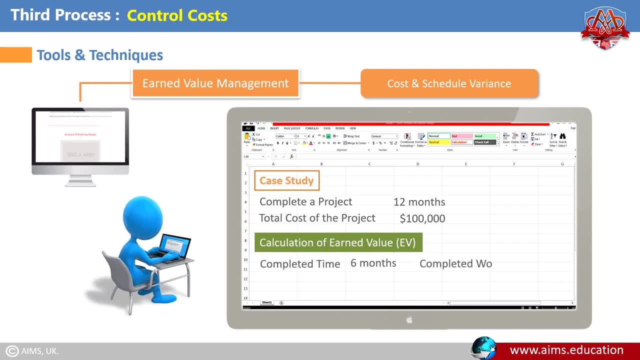 that you've spent $60,000, but were able to complete only 40% of the project work. So the earned value of the project will be calculated as Earned value equals 40% multiplied by $100,000, Or earned value equals $40,000.